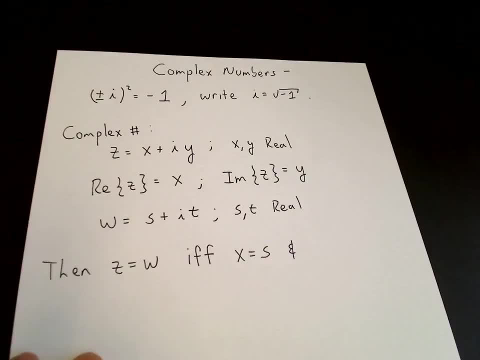 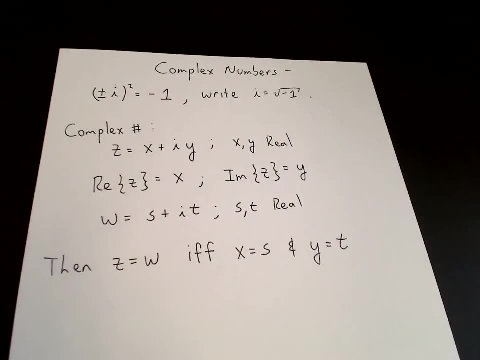 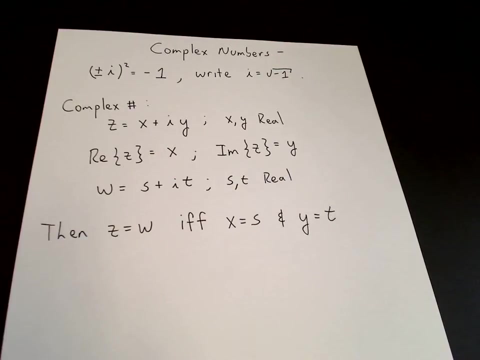 and the imaginary part of z is equal to the imaginary part of w. y is equal to t. So one complex equation, z equals w, is equivalent to two real equations. The real part of the left-hand side equals the real part of the right-hand side. 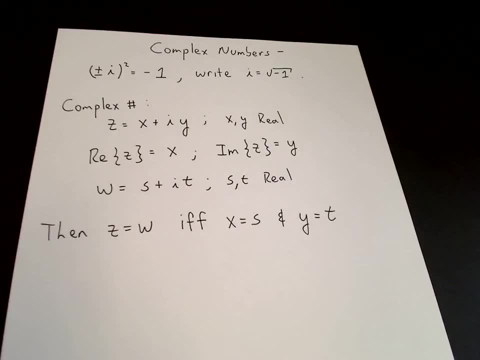 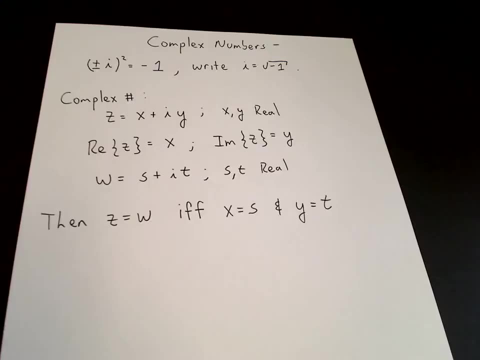 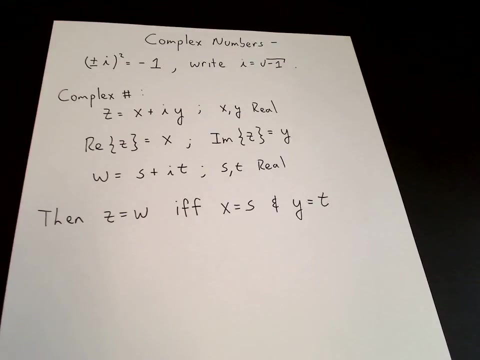 and the imaginary part of the left-hand side equals the imaginary part of w. Okay, a nice thing, property of complex numbers is that if you add two complex numbers, you get a complex number. If you multiply two complex numbers, you get a complex number. 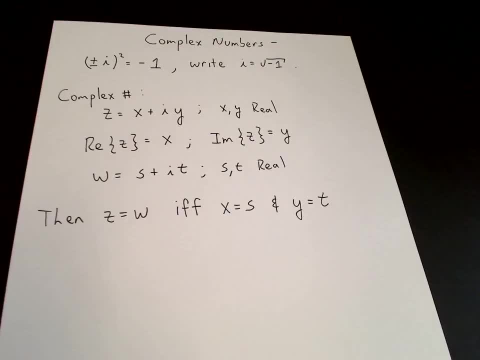 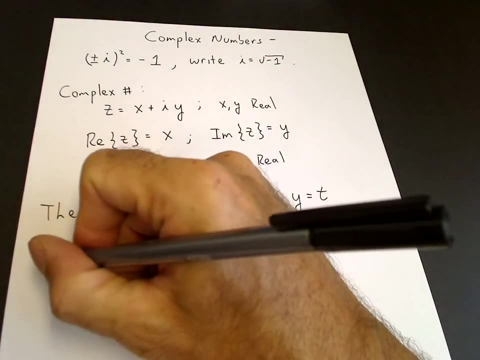 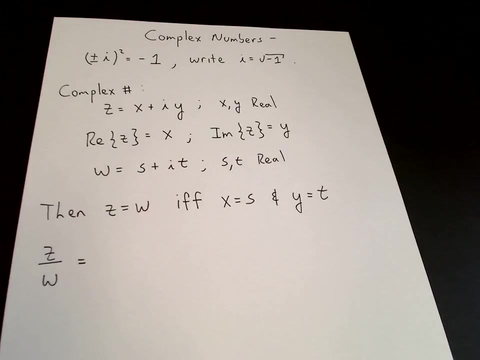 If you divide two complex numbers, you get a complex number. Division is the hardest one to see, so let's work it out. So if we divide two complex numbers- z divided by w- to show that this is a real equation and this is a complex number, we have to write that as a real part, plus i times an imaginary part. 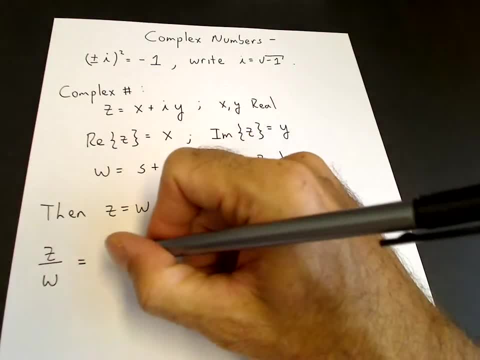 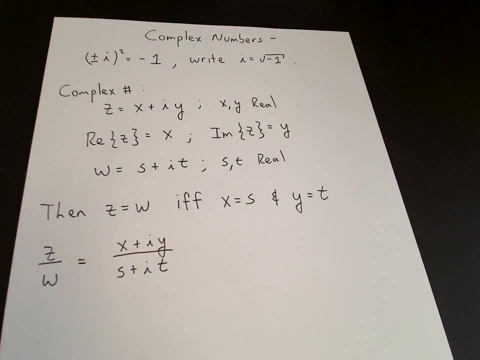 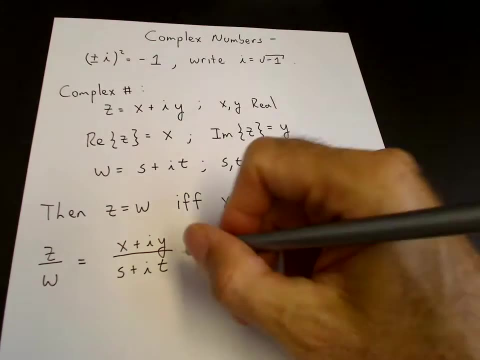 So this is x plus i y divided by s plus i t. So in this form it doesn't look like a real part plus i times an imaginary part. But we can make it look like that by multiplying by 1, where the 1 we write as the denominator. 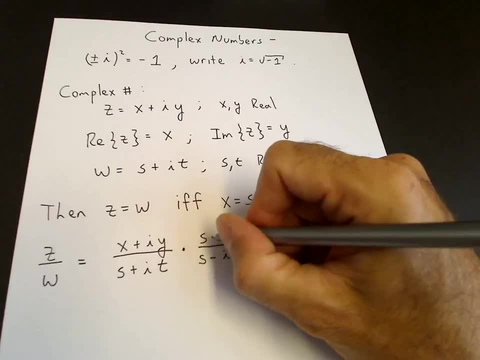 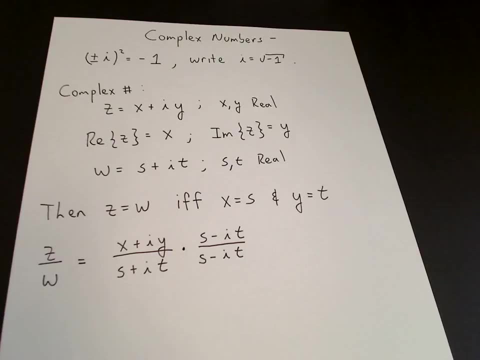 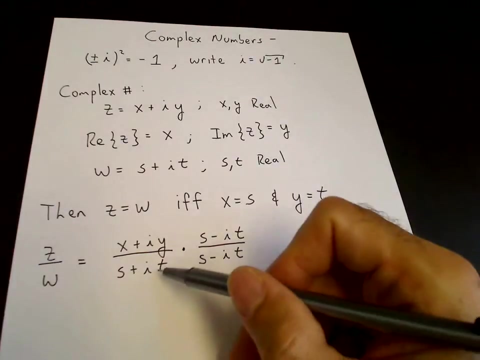 has in the form s minus i t, so the numerator is the same, And when we do that, we have the nice property that s plus i t times s minus i t is s squared plus the cross terms, which exactly cancel because they're opposite sign. 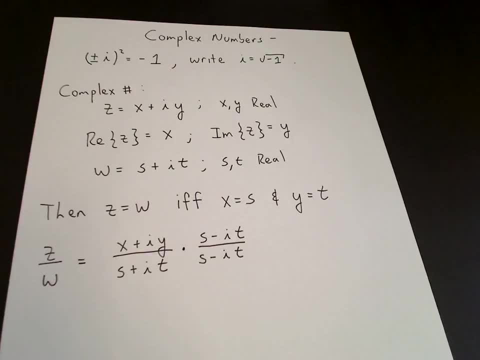 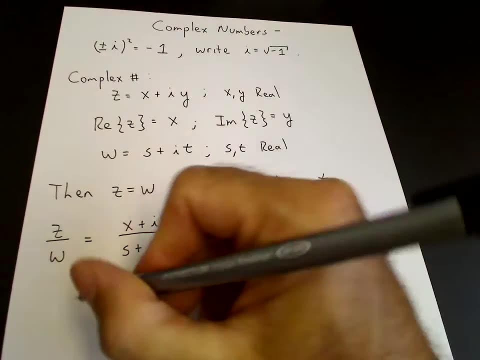 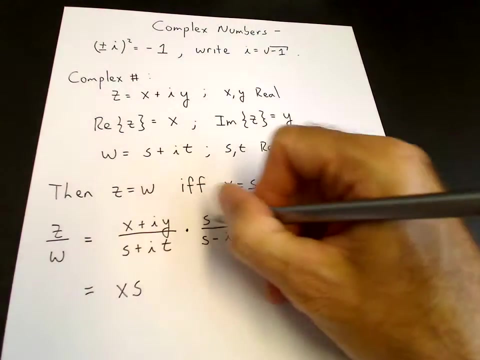 minus i squared times t squared, and i squared is minus 1.. So the denominator is s squared plus t squared, Which is real, And then we can collect the terms of the numerator. So the real part of the numerator will be xs. the cross terms will be imaginary. 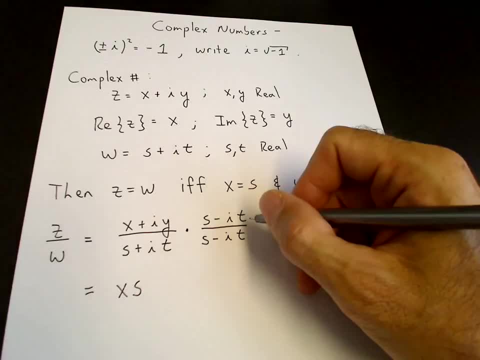 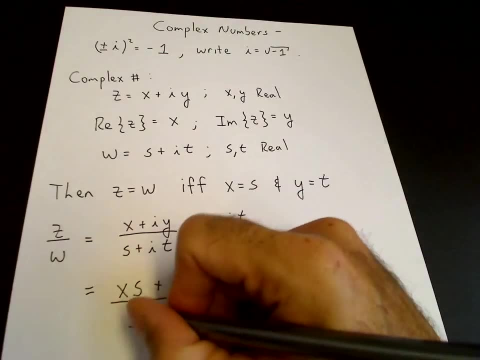 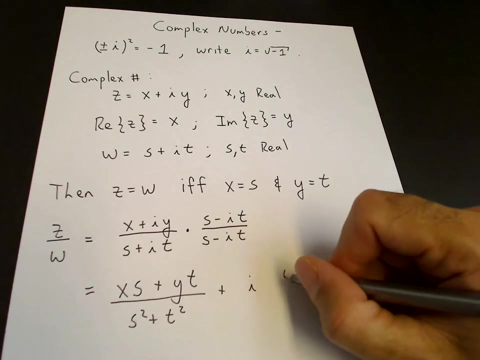 and ey times minus. it is minus i squared plus 1 times yt. Xs plus yt divided by the numerator, which is s squared plus t squared plus i times the cross term of xs and yt, And then we have our numerator, which is now more than that. 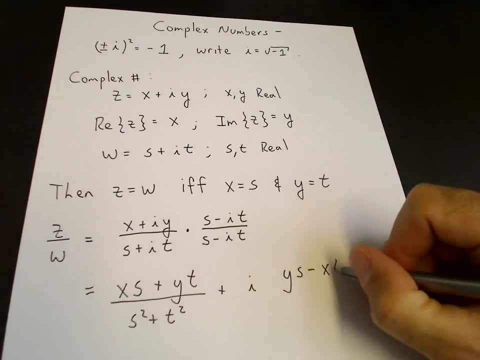 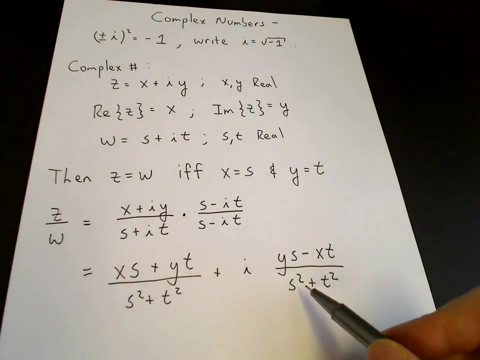 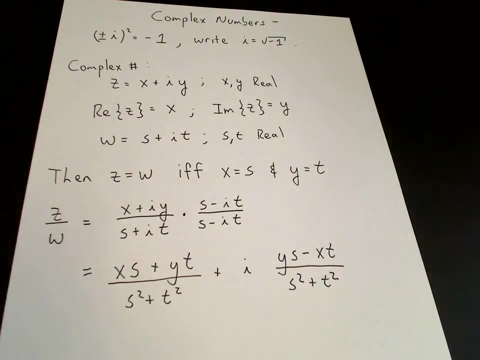 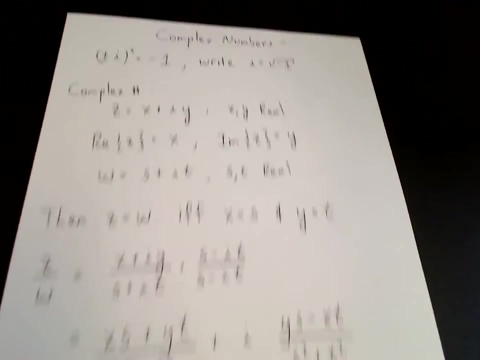 the numerator divided by the denominator. So now we've written the division of two complex numbers by a real part plus i times an imaginary part which is a complex number. This multiplication of s plus i t by s minus i t is rather special, and we introduce that as a new function which is called 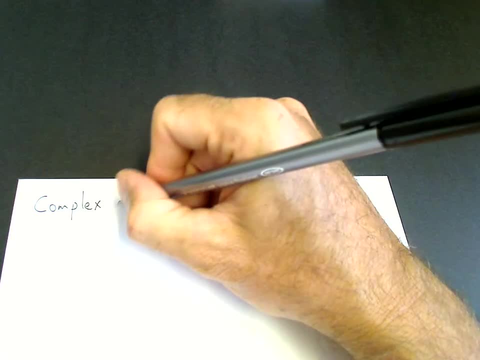 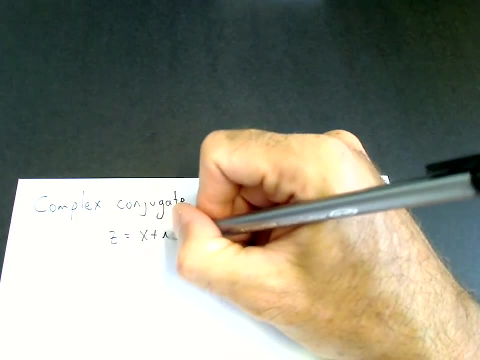 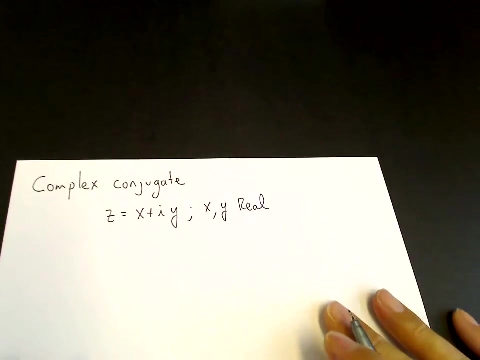 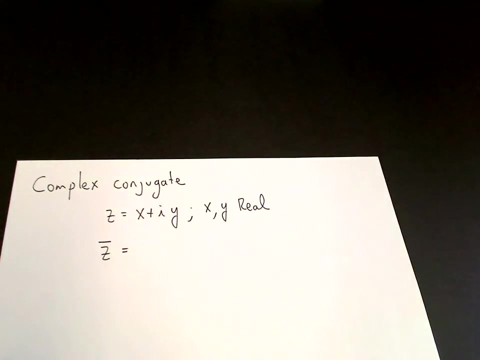 the complex conjugate. So with z equals x plus i, y, x and y are real. We define the complex conjugate of z- z bar as change the sign of the imaginary part. So x minus i, y, The complex conjugate has. 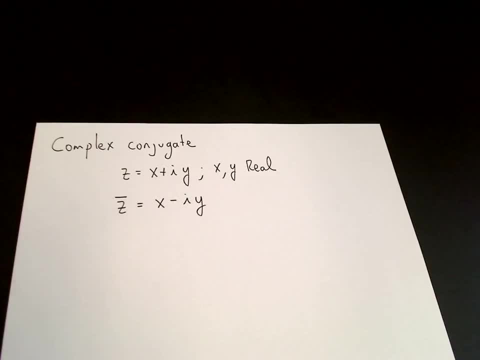 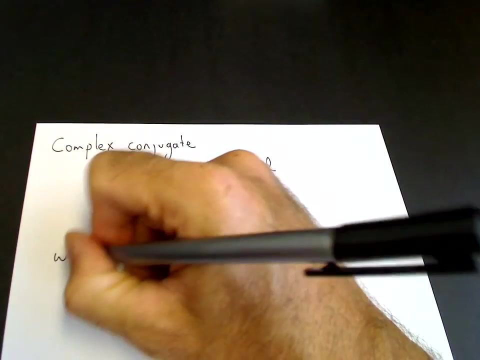 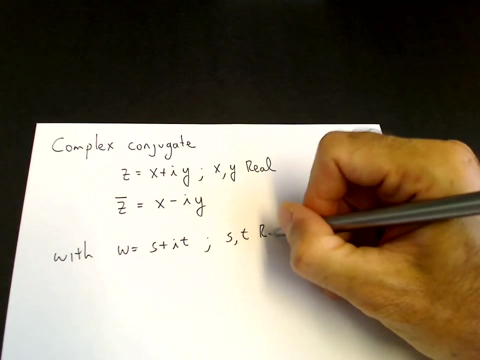 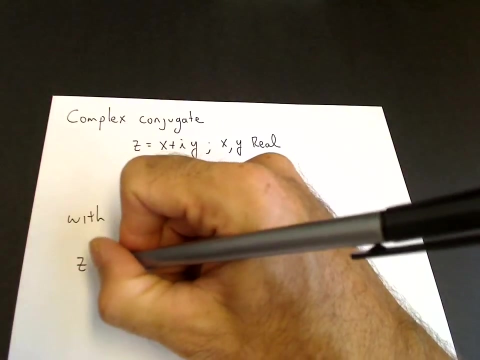 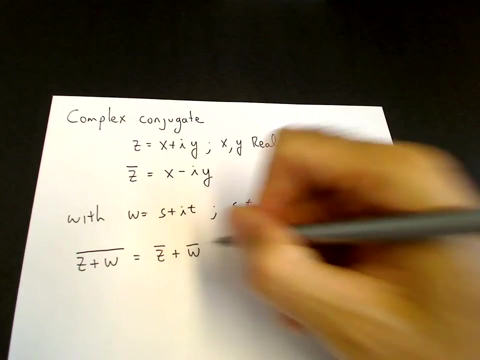 a nice property that the complex conjugate of the sum of two complex numbers is the sum of the complex conjugates. So with w and a small 훨씬, the complex conjugate of the z of w equal to the x plus i t, Z, bar for the. 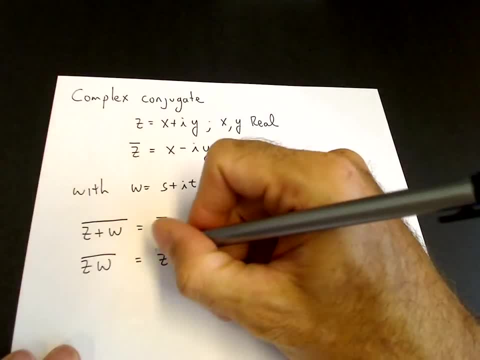 z bar per union room We get a Articulate of the complex conjugate of z. So that's anything más or minus the rule worth, if we take that real, so that we haven you know n o v. This is the complex conjugate of z. times keeps dulibh完. 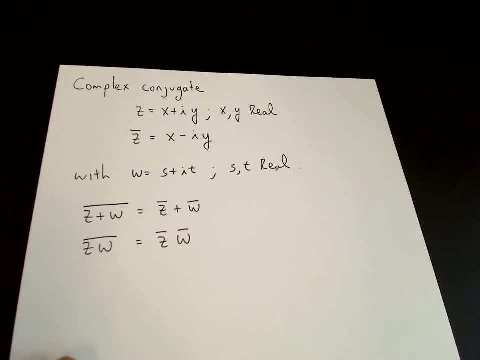 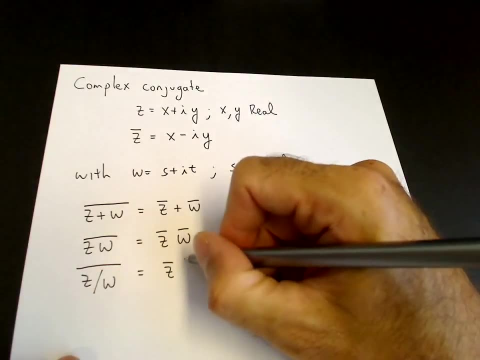 s n t and here, when you do that and you get that number- and this is something else- times the complex conjugate of w and the complex conjugate of z divided by w. is the complex conjugate of z divided by the complex conjugate of w. 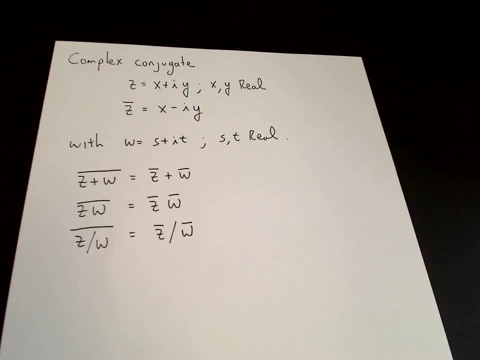 So when you have a complicated, complex expression with i's in a lot of different places, with real numbers, real variables scattered about, possibly with complex variables scattered about, if you want to take the complex conjugate of that expression, then i's become minus i- real variables don't change. 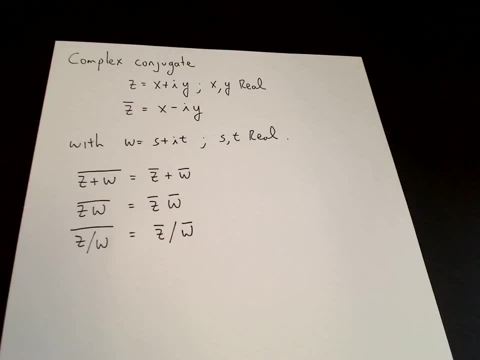 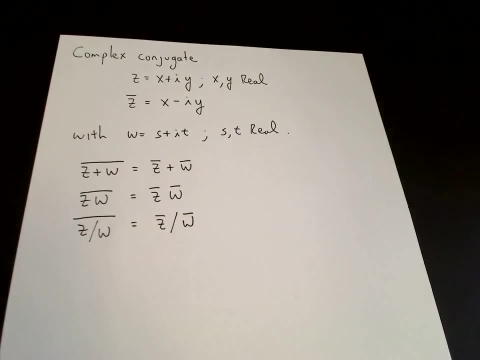 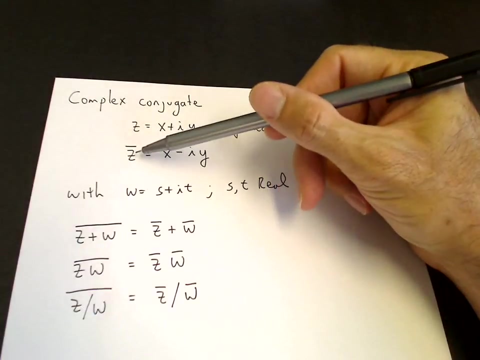 complex variables become the complex conjugate of the complex variables. That's what these relations tell us. And it's useful to do complex conjugates Because if z turns out to be a real variable, so if you want to impose a condition on z such that z is real, 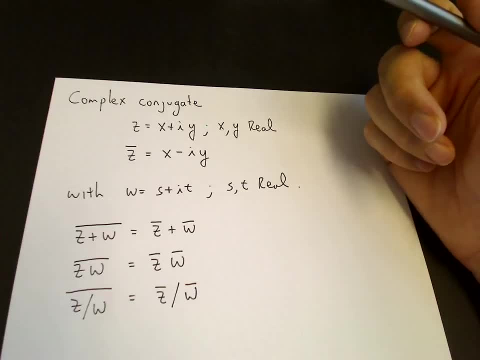 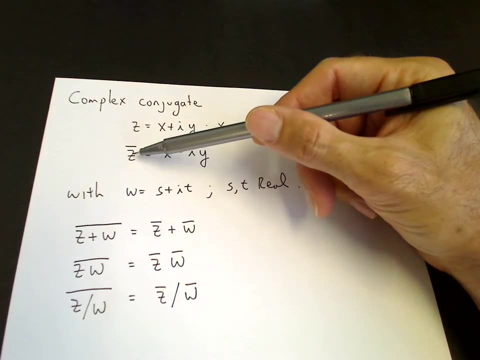 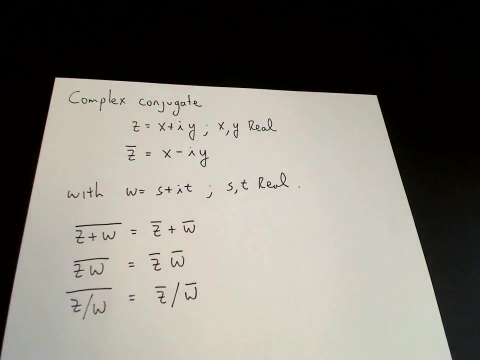 the equation that expresses that imposition could be imaginary. part of z equals 0, but it could also be simply that z is equal to z-bar, its complex conjugate. If z equals z-bar, then y has to be 0,, z has to be real. 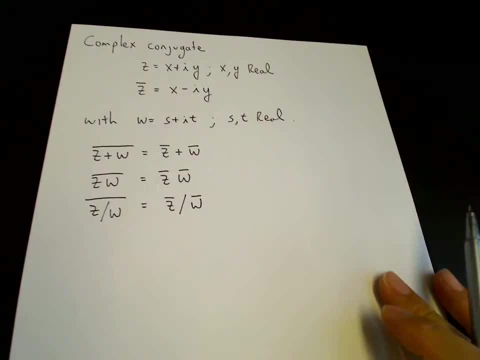 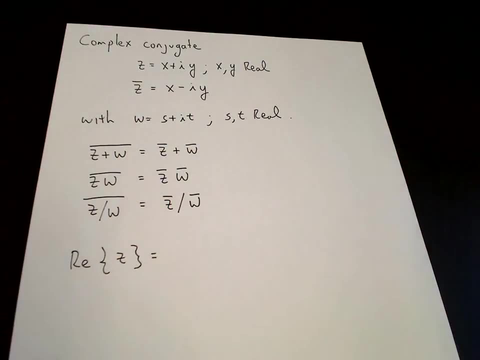 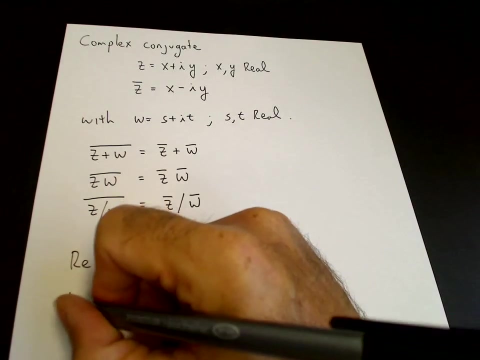 It also gets a little bit complicated. It gets a way of getting the real part of z right. So the real part of z is just summing z and z-bar and taking one half of that sum right, And the imaginary part of z is derived from the distance, the difference. 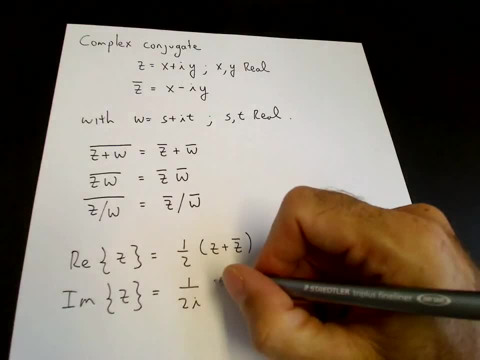 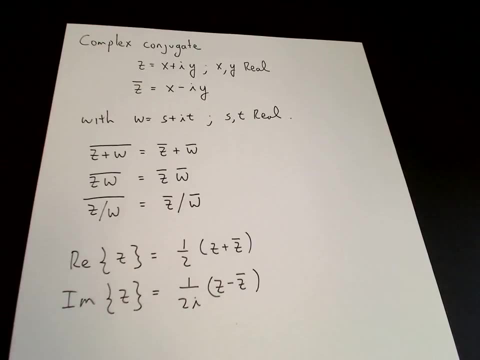 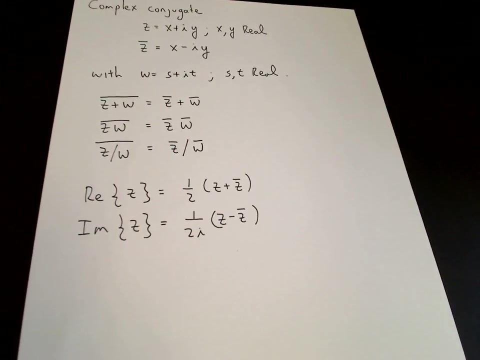 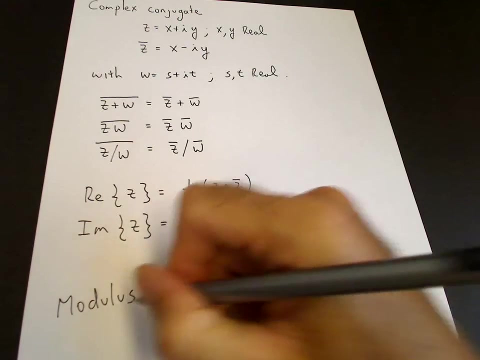 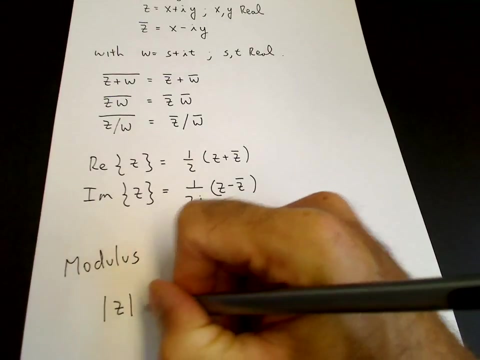 So 1 over 2i times z minus z-bar will give us the imaginary part, And those are also very useful relationships. The other useful new function in complex variables is the modulus of z. So we define the modulus of z using the absolute value sign. 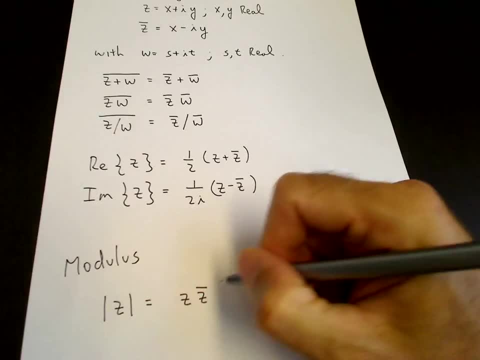 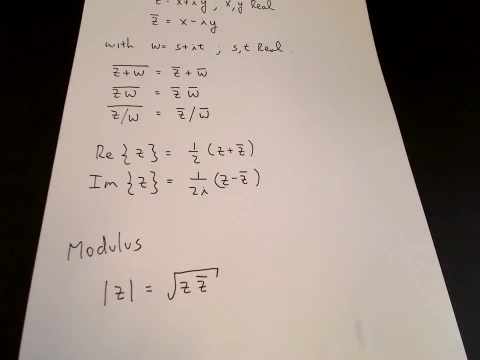 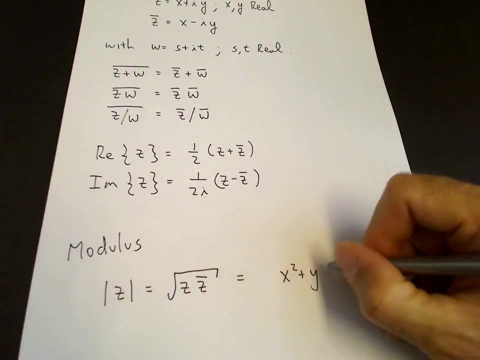 as z times its complex conjugate, times its complex conjugate square root right. And if z equals x plus iy, we've already shown that z times z-bar is x squared plus y squared, the real part squared plus the imaginary part squared. 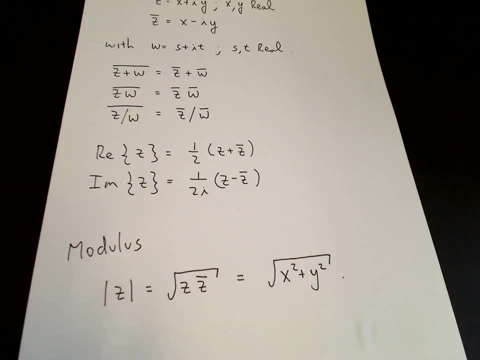 and we take the square root. Okay, In the next video in this complex number series, we'll then talk about exponential function.